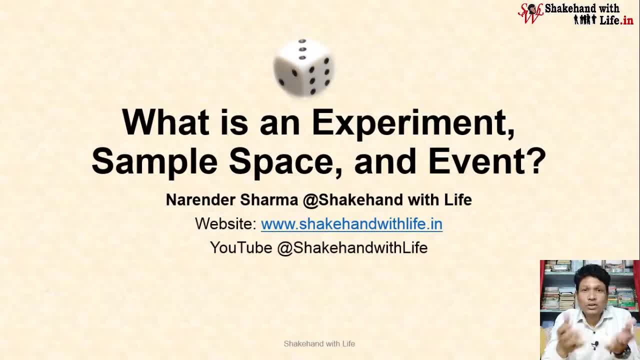 Hello everyone, Welcome again to this new episode of Shake Hand with Life. I am Narendra Sharma And in this video I am going to tell you about some basic concepts of probability. So here I have an experiment, sample, space and event for you. These three basic concepts of probability are very important to study the probability, to understand the concepts of probability Right. So let's start with an experiment. 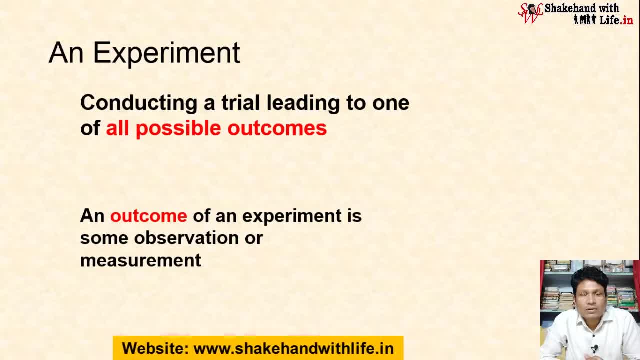 So what is an experiment? An experiment is conducting a trial leading to one of all possible outcomes. When we conduct an experiment, we have number of possible outcomes, So therefore, conducting a trial leading to one of all possible outcomes is an experiment. Then what is an outcome? 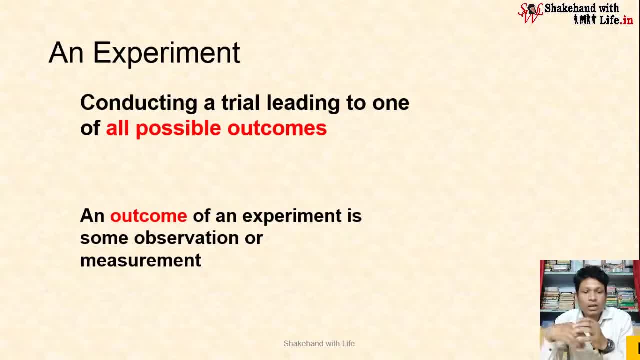 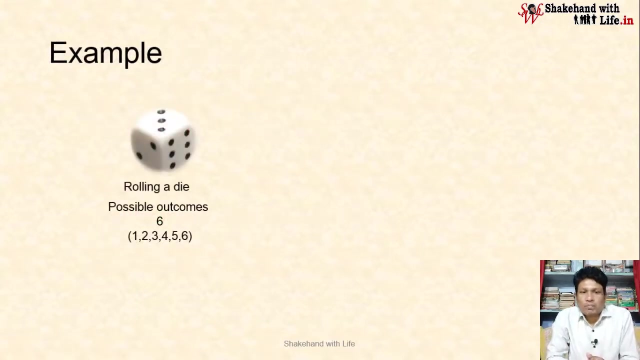 An outcome of an experiment is some observation or measurement. This is the outcome. When we observe something as a result of an experiment, we have an outcome. Right? Let's take some examples to understand the experiment. Okay, Here, if we roll a die, then 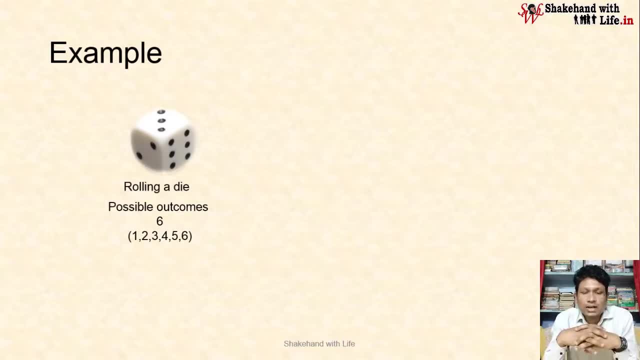 we have six possible outcomes, Right. And what are these six possible outcomes? One, two, three, four, five and six? We have any one number out of these six possible outcomes Right? Take another example: Drawing a card is an experiment. 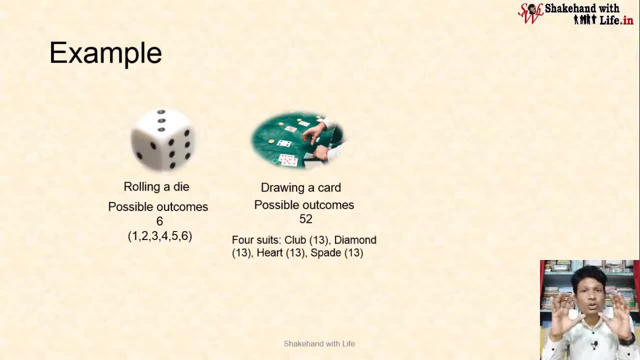 When we draw a card, we have 52 possible outcomes. Either we have a card of club, any number of club, any number of card of diamond, any number of card of heart, any number of card of spade. We may have any card out of 52. 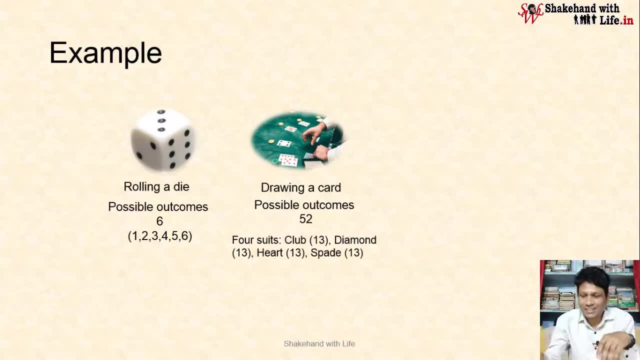 possible outcomes. So this is an experiment, Right? Similarly, when we toss a coin, we have only two possible outcomes: Either we have head or we have a tail. Only two possible outcomes are there, Right? So this is an experiment. Now let's talk. 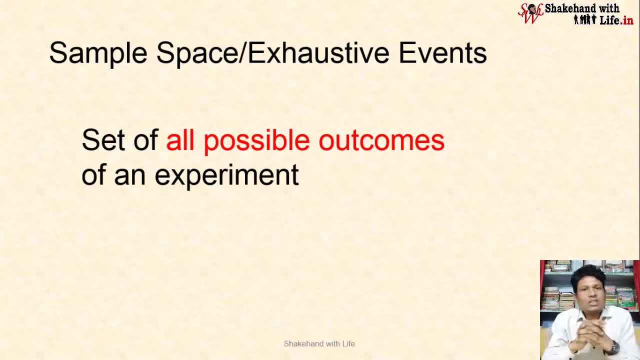 about the sample space. What is a sample space or exhaustive events, A set of all possible outcomes, a set of all possible outcomes of an experiment. When we collected all possible outcomes of an experiment, we have a sample space or exhaustive events. Now let's take some examples to 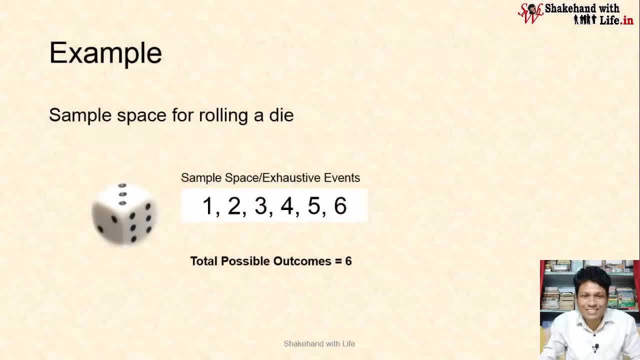 understand the sample space or exhaustive events, The sample space for rolling a die. When we roll a die, then what is the sample space? We have one, we have two, three, four, five and six. These are the possible outcomes. So this is. 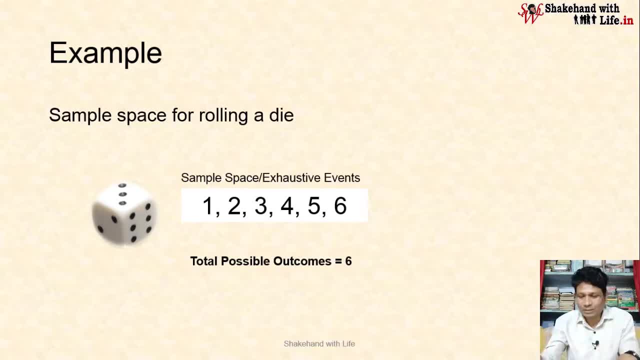 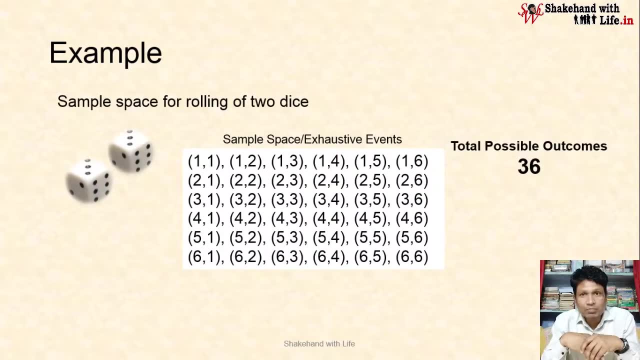 the sample space for rolling a die Right. Six possible outcomes are there. Similarly, when we roll two dice simultaneously, then what is the sample space? So here we have the sample space. This is our sample space. First die may have one, then second die may have one. 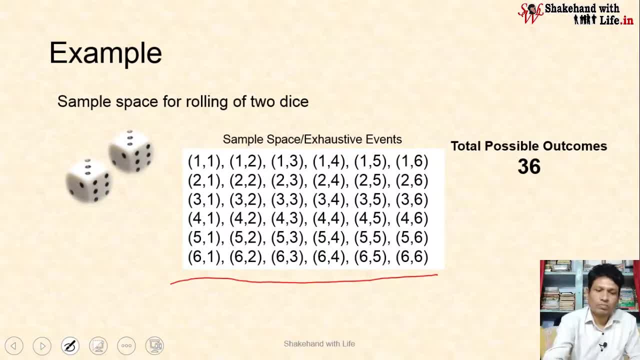 two, three, four, five and six Right. Similarly, first die may have two, then the second die may have one, two, three, four, five and six, And in the same way we have thirty total possible outcomes when we roll two dice. 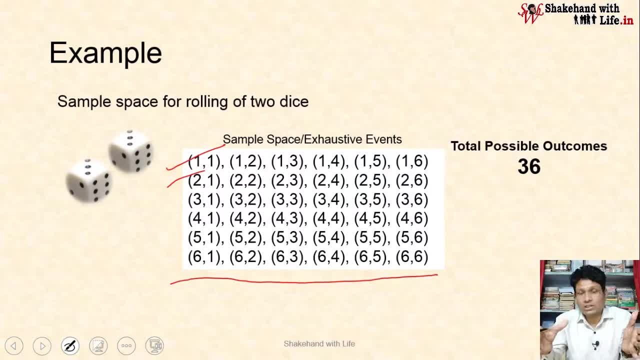 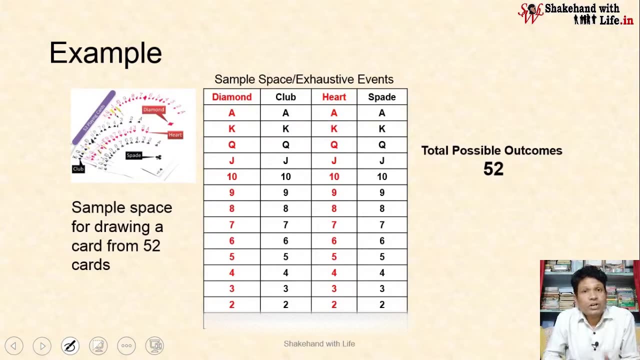 simultaneously Right. So this is the sample space: Collection of all possible outcomes, or set of all possible outcomes. is the sample space Right Now? similarly, when we draw a card out of fifty two cards, then what is the sample space and what are the exhaustive events? 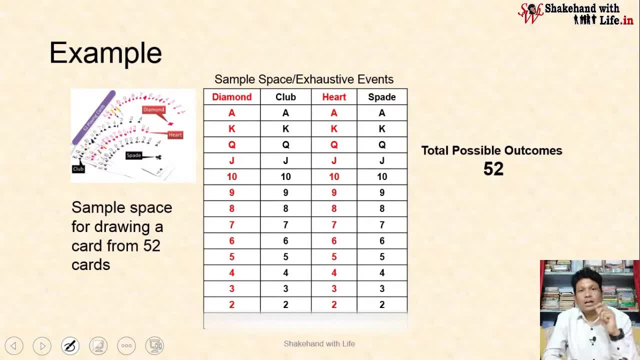 So when we draw a card, then it may be any number card or any suit of card Right. It may be a number of card of a diamond, it may be a card of club, any number of club. It may be a card of heart, It may be a card of. 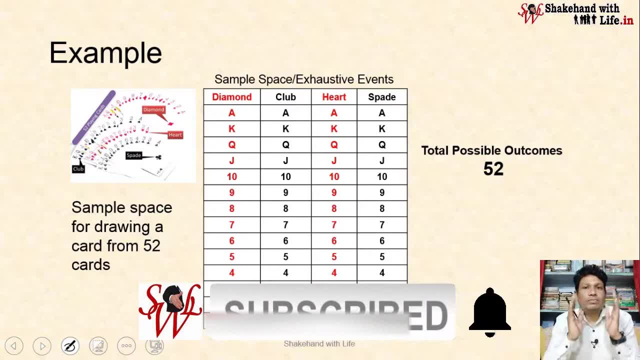 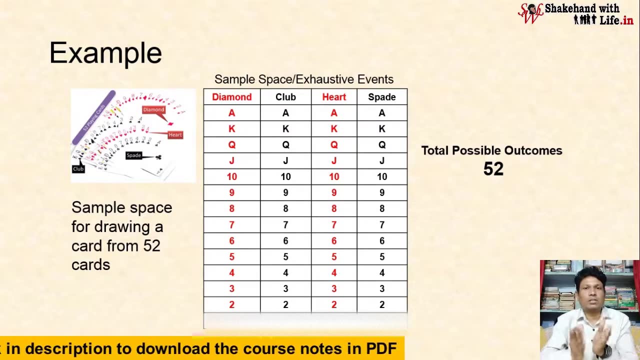 spade. So we have fifty two possible outcomes, And we may have any card when we draw a card. So the sample space is thirteen card of diamond plus thirteen card of club, plus thirteen cards of heart plus thirteen cards of spade. Right, This is our. 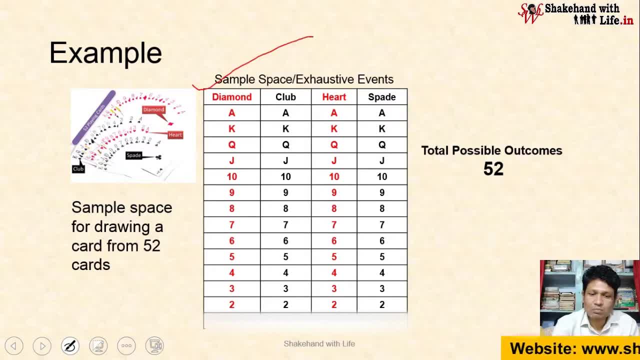 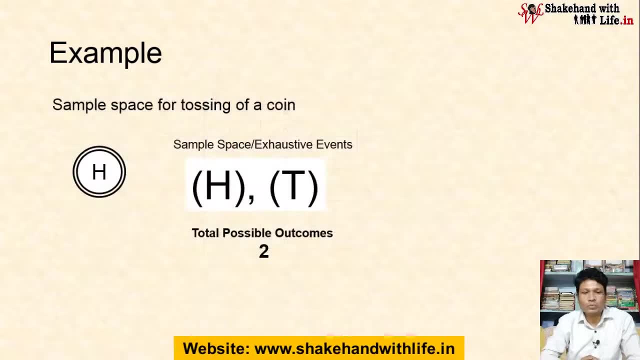 sample space. So this is our sample space. This is the sample space, Right? Okay, Now what is the sample space? when we toss a coin, We have only two possible outcomes. So the set of two possible outcomes is the sample space Either we have. 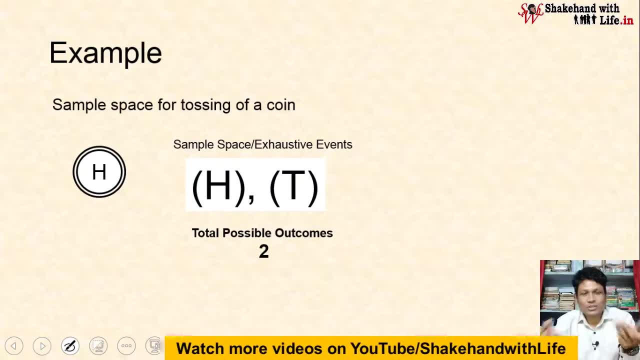 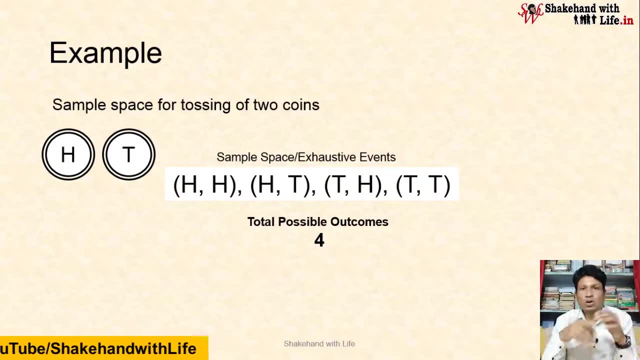 head or we have a tail. So this is the sample space for tossing a coin. Now, what is the sample space for tossing of two coins simultaneously? So here we have the sample space. First coin, head. Second coin is also head, Right. 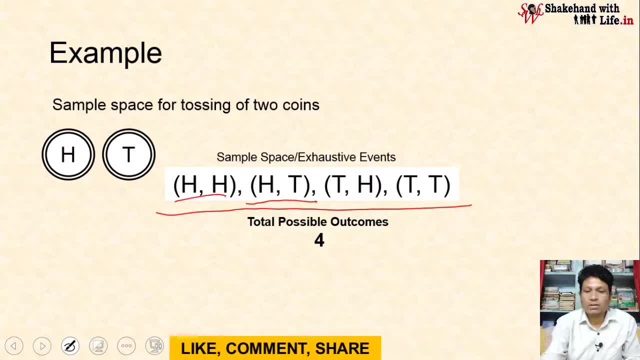 First coin head, Second coin has tail. First coin tail, Second coin head. First coin tail. Second coin also be tail. So this is the sample space, All possible outcomes, A set of all possible outcomes, Right? So these were the examples of 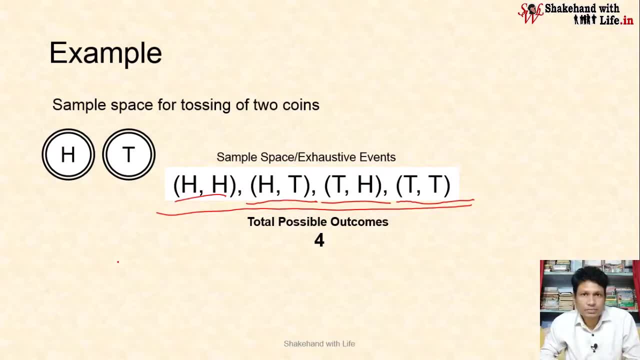 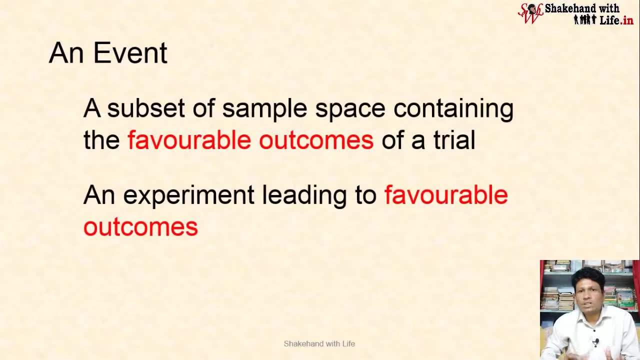 sample space or exhaustive events related with an experiment. Okay, Now we understand what is an event: A subset of a sample space containing the favorable outcomes of a trial. When we do some experiment, we have total possible outcomes for an experiment. But if we 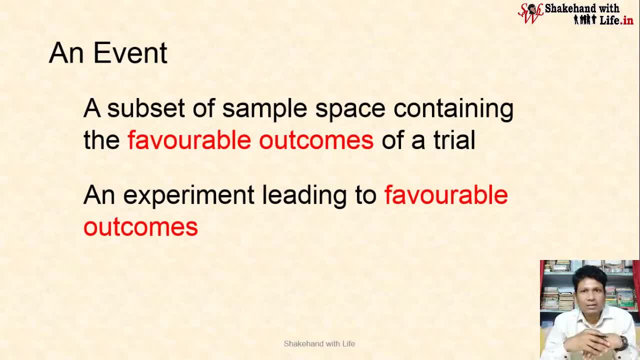 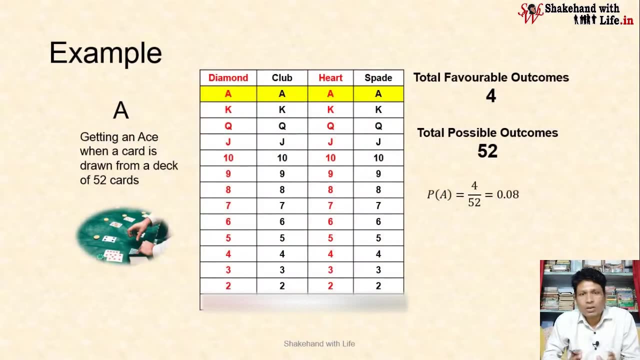 have some favorable outcomes for a trial, then we have an event. That's why we can say that an experiment leading to favorable outcomes is an event. Right Now we understand, with some examples What is an event. Let's say A is an event. 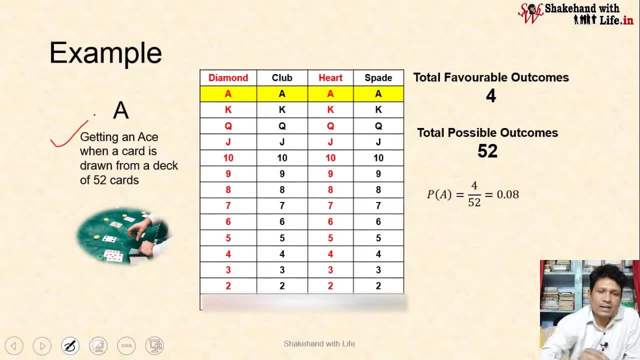 And what is that event? Getting an ace when a card is drawn from a deck of 52 cards. Getting an ace Right. So the total favorable outcomes: we have four favorable outcomes Right. These are the four favorable outcomes: Ace of diamond, ace of club. 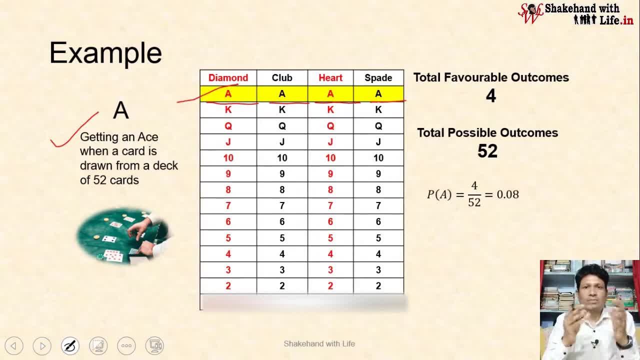 ace of heart, ace of speed. These are the four favorable outcomes And we have the sample space for this experiment: 52 possible outcomes. Right, That's why the probability of this event- that means getting an ace, the probability of getting an ace- is PA equal to. 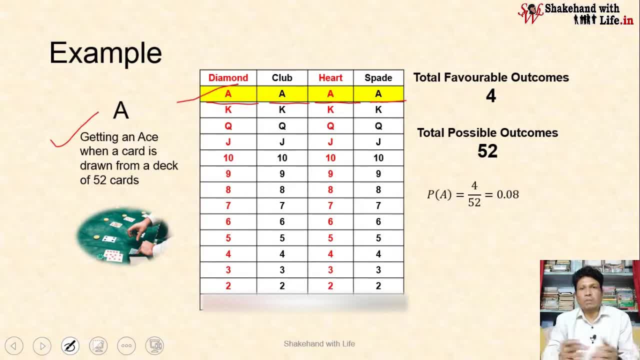 4 divided by 52 and we have 0.08. that means 8 percent. That means we have 8 percent probability that we may get an ace when we draw a card out of 52 cards. Right Another example we have B is an event. 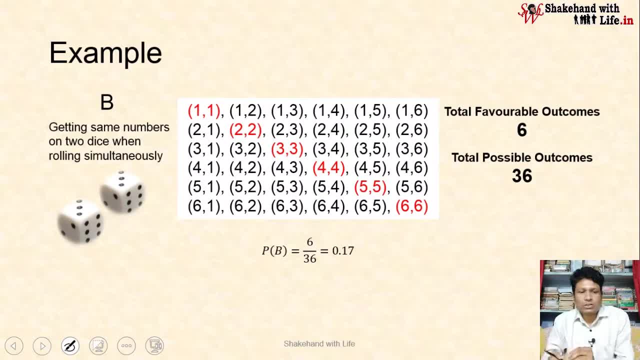 which says that getting some same numbers on two dice when rolling simultaneously. This is an event And the favorable outcomes are 6 only. And what are these outcomes? These are 1-1, 2-2, 3-3, 4-4. 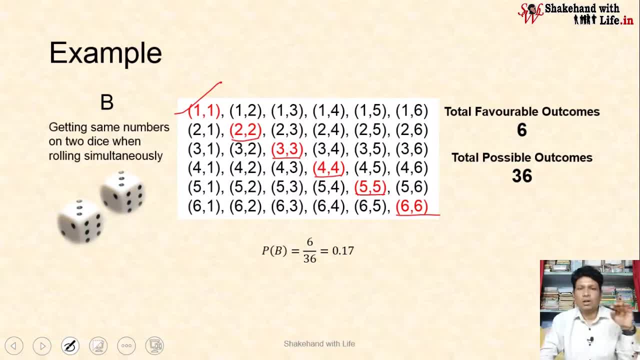 5-5, 6-6. That means, first die has 1,, second die also has 1, first die has 2, second die also has 2, and similarly 1-1, 2-2, 3-3, 4-4, 5-5. 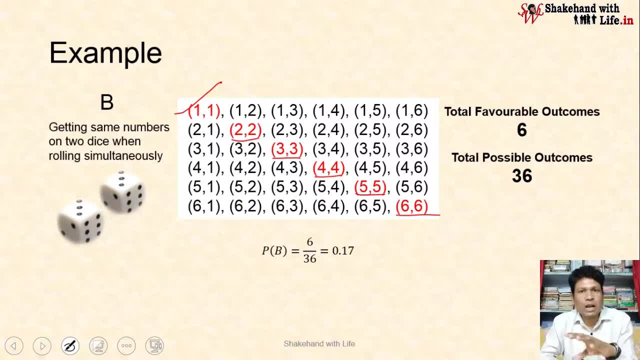 and 6-6.. 6 favorable outcomes Right, And the total possible outcomes are 36.. We have the sample space for that. Now the probability of getting the same number on two dice. we have PB equal to 6 divided by 36.. PB is: